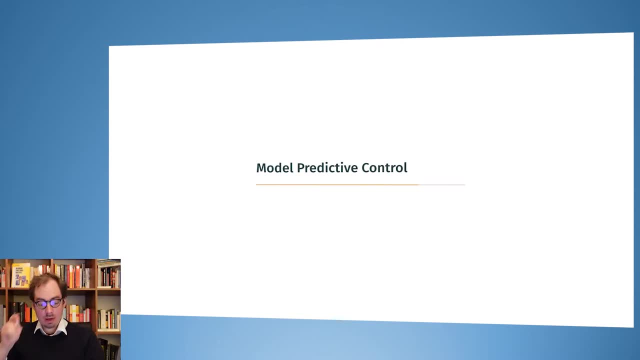 time and moving randomly. And now our example is concerned with numbers in space and time control. And this is interesting if, for example, you want to go into robotics or if you want to control physical systems, because now we will learn how to take a system and make it behave. 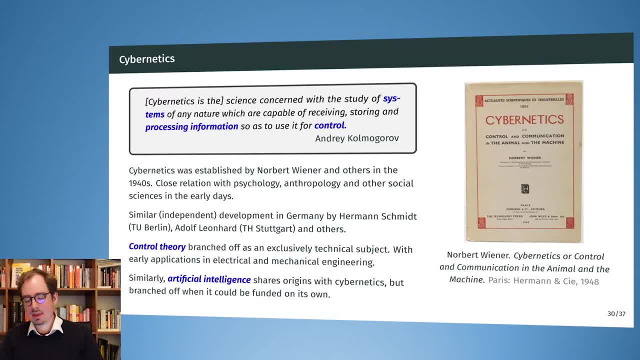 in a way that wouldn't be natural, And the example that we are using here is the inverted pendulum that we also saw in the first equation at first lecture. Now some history: The control theory that exists today is a development that was started or is the outcome? 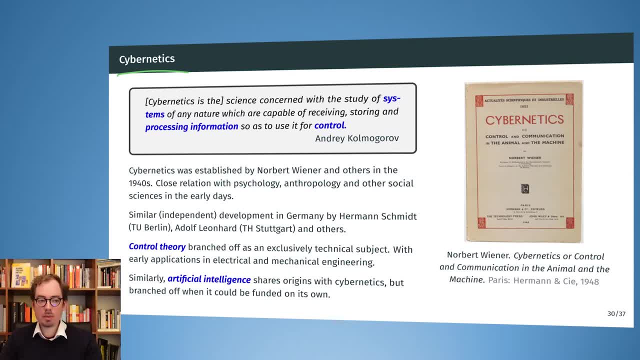 of a development started in the 1940s which back then has been called cybernetics. So Norbert Wiener is the father of cybernetics, or he coined the term cybernetics in his book. cybernetics or control and communication in the animal and the machine. So groundbreaking book and 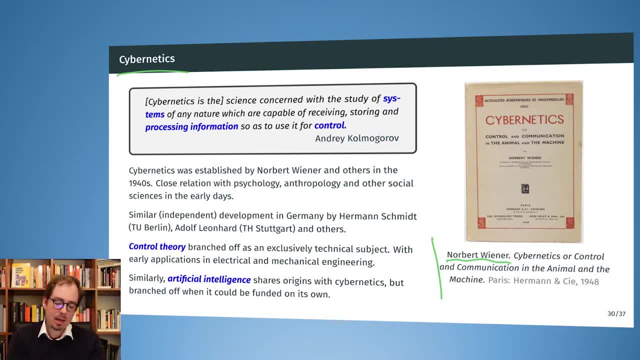 this was considering feedback mechanisms And Andrei Kolmogorov, a very famous researcher. he called cybernetics the science concerned with the study of systems of any nature which are capable of receiving, storing and processing information so as to use it for control. 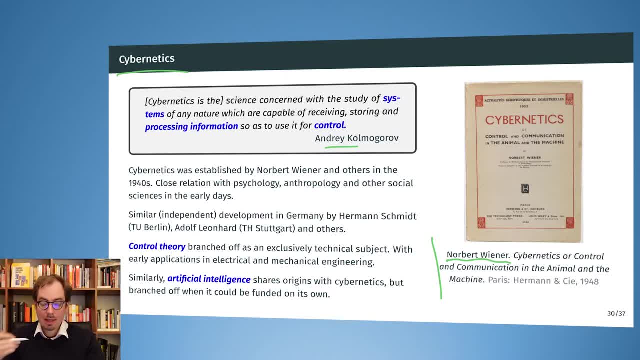 And control can be many things. So control can be a rocket going to the moon. control can be a car staying in the middle lane. Control can be the inverted pendulum swinging up. Control can also be an electrical in an electrical motor, or a chemical plant or a biological system. So somehow, 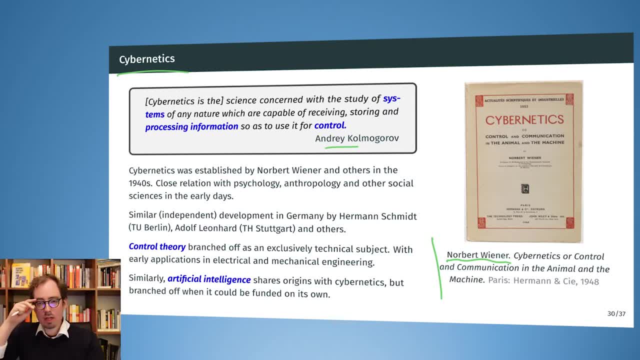 a system that is self-regulating by receiving information and using it to change its future state, So cybernetics founded in the 1940s. Back then, this was a mixture of many fields, including computer science, computer science and computer science. 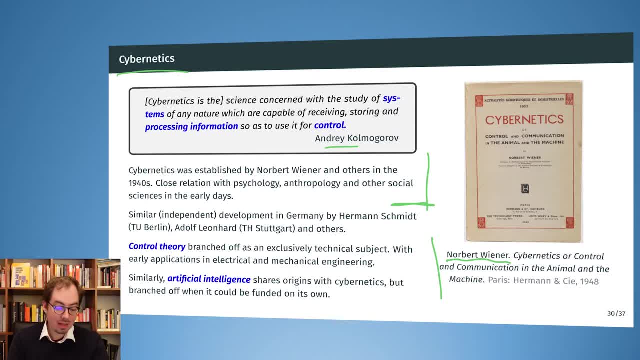 computer science and computer science, And they were also interested in feedback mechanisms, not only the technical sciences, but also psychology, anthropology and many others. Besides the development in the US, there was also an analog development independently in Germany by Hermann Schmidt, Adolf Leonhard Rudolf Oldenburg and a couple more. 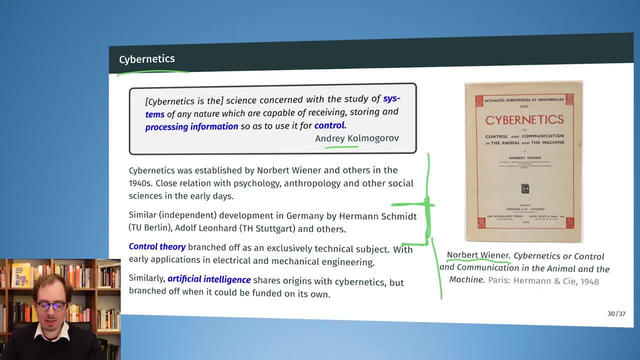 And this is how cybernetics- how to say, stream from the US- is the more prominent one, And control theory. control theory as it is considered today by electrical engineers or by mechanical engineers, is essentially branched off from the original cybernetics term. 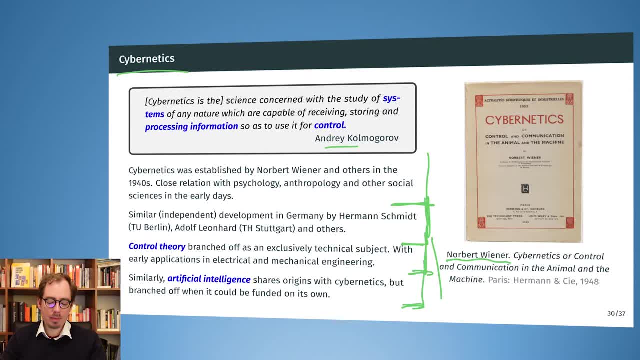 In Stuttgart you can still study technische kybernetik. but again, essentially this is today control theory. When we talk about cybernetics in a methodological sense, this is essentially a control theory. It is a mathematical term, in a systems term and no longer also in a psychological or anthropological. 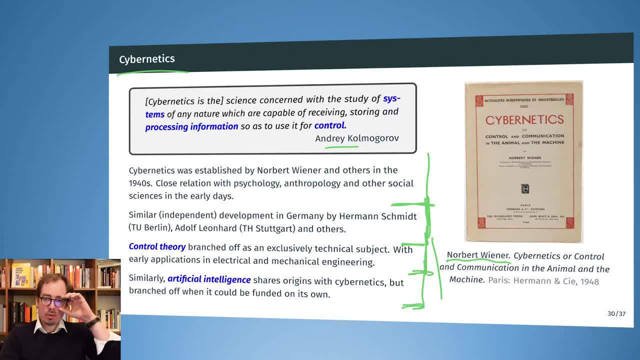 social sciences way. Some of the early researchers in artificial intelligence have also been there in the cybernetics community. but after the famous Dartmouth symposium or the conference in Dartmouth, they also branched off and got funding on their own and also got their own brand then for doing. 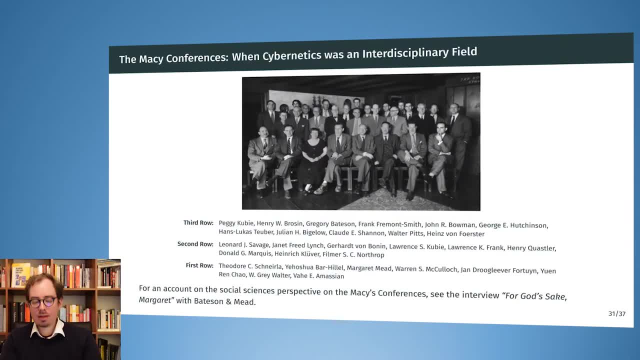 you know, artificial intelligence. This is an interesting picture. So this is a picture from the Macy conferences. I think they started in like 1942 or something, And this was a yearly conference where the researchers in cybernetics came together, And this is just a who is who of famous, famous researchers at the time. 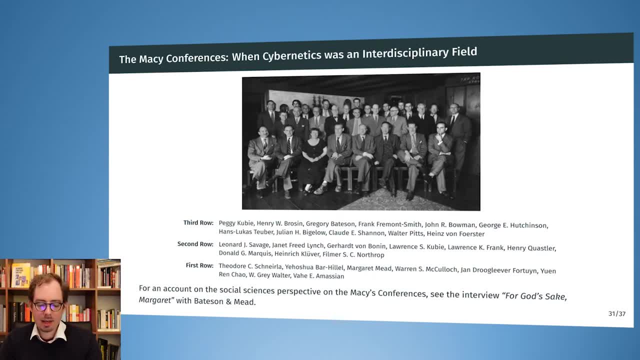 So you had John von Neumann, You had Norbert Wiener, You had, like, Pitts and McCullough, So the guys who invented the neural networks in the 40s and 50s. So I think Pitts is, Pitts is, this is Pitts and McCullough is, I think, in the second. 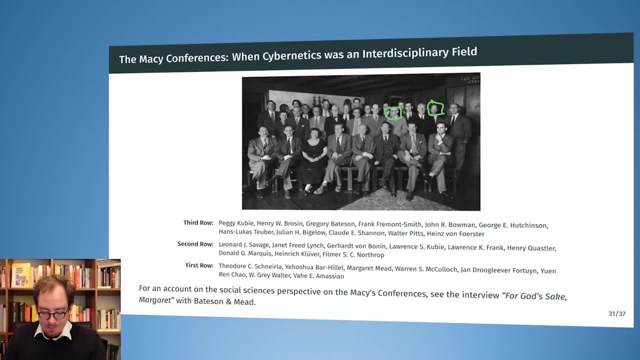 line somewhere, No, in the first row, I'm sorry. So McCullough is, that's McCullough. So these were the inventors of the neural networks. But mixed into that, into the famous mathematicians, oh, somewhere there's even there's Claude. 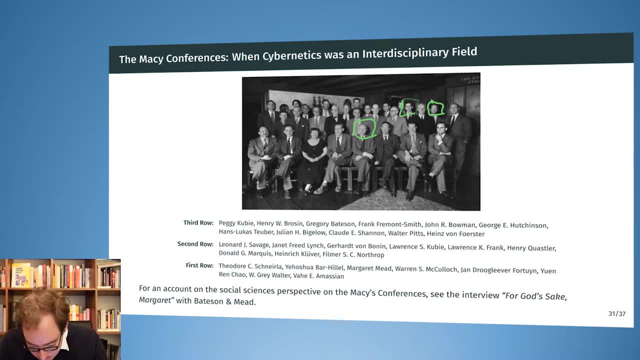 Shannon. Where is he? Claude? this is Claude Shannon. So if you haven't read A Theory of Communication, you must. It's a very readable paper and it advanced humanity by at least 10 years, And so mixed into these very famous researchers that were more mathematicians. 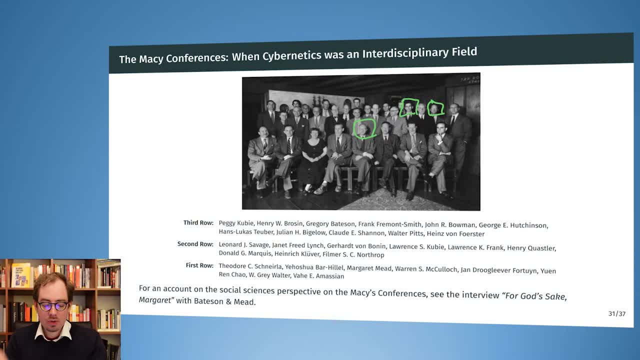 So yeah, Yeah, Yeah, If you're more mathematically inclined, you also had very interesting people from the social sciences, So, for example, Margaret Mead and Gregory Bateson, and these were very interested also then in feedback mechanisms, in the human 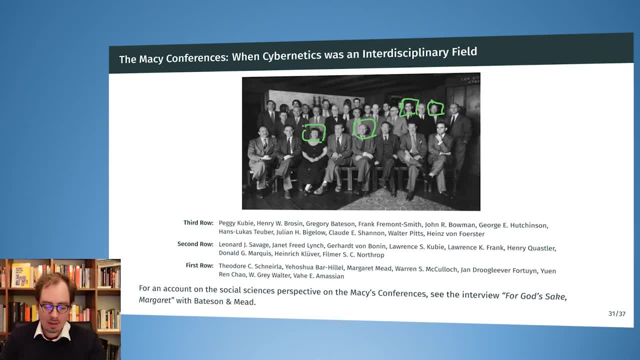 For example, even the term, the word feedback- it comes from this Macy conferences. They invented it back then. Before this, this concept didn't really exist. And so today, a boss that that was sent to enough corporate trainings and then he knows that he has to give. 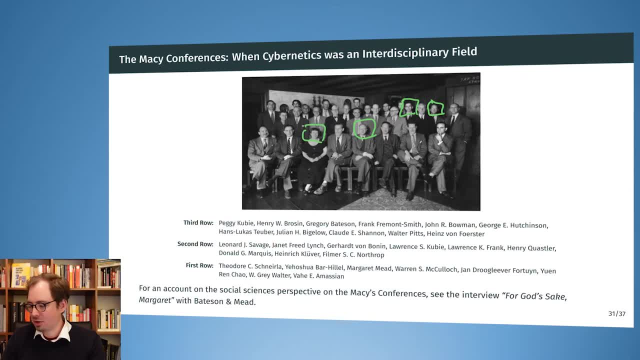 you feedback and he, he packages it as a, as a sandwich, where he says something nice in the beginning and at the end. um, so the word feedback and how that works it, it took its origin at the macy conference and at the same conference they talked about very deep mathematical. 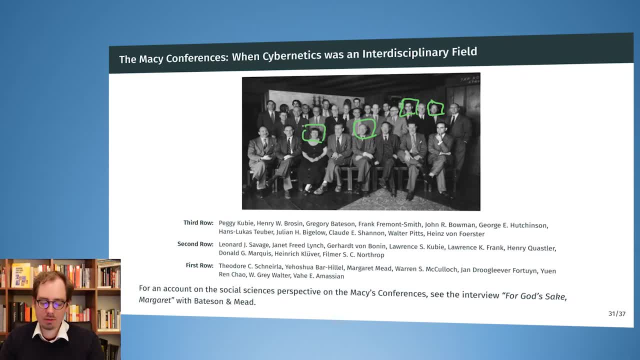 subjects that led to to control theory that we have today. and uh, it's even more strange than that because in the early days at the macy conferences, they were interested in in subjects like hypnosis, but because they were serious researchers, serious researchers, they couldn't say hypnosis, so they 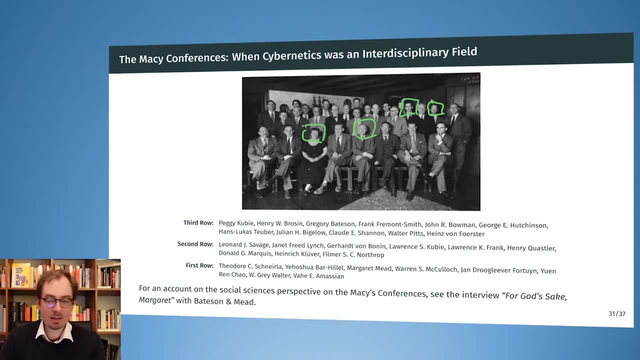 had to use different words for the effect in order to to be respectable, and uh, margaret means, for example, she went to bali and to see how people went into trances and used hypnosis in daily life and crazy things, and so this was a really a hotbed of interesting new ideas. and then, after some time, the, the social, 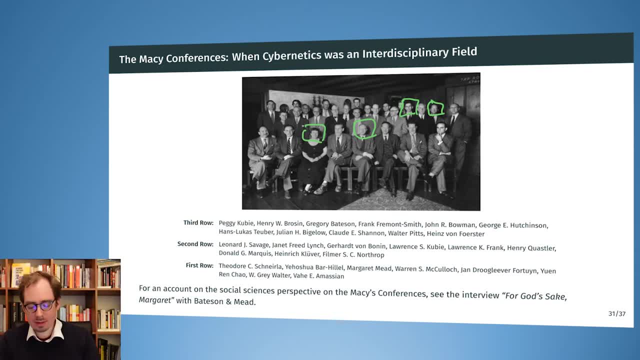 sciences and mathematical sciences. they they somehow separated. but we still have a lot of effect today from these macy's conferences, and there's an interview with margaret mead and gregory bateson that that shows this other perspective. on on on the macy conferences. okay, but now to the actual content. 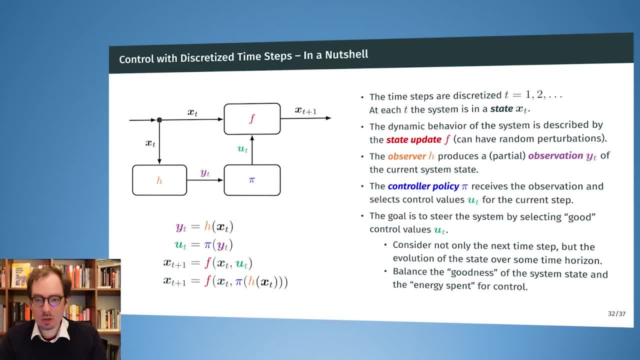 so, um, we're back and we are now doing some control theory, so it's all pretty basic, but in the end we can still control a physical system to do something that it wouldn't normally do. what we see here depicted is a high level overview on control. 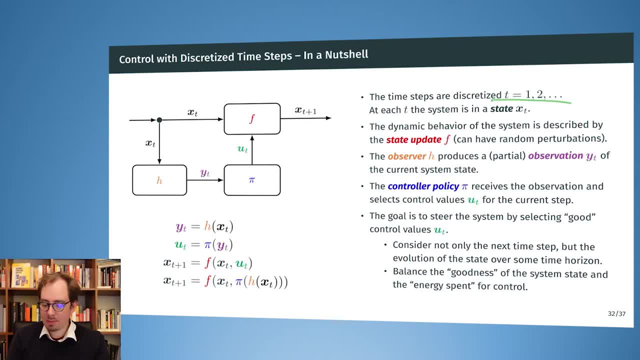 so, uh, we have discretized our time step. this is one of the first assumptions that we are making. we have discretized our time steps. so, and then we have like a hundred milliseconds or so in between our discrete time steps that we are considering and the system that we have, the 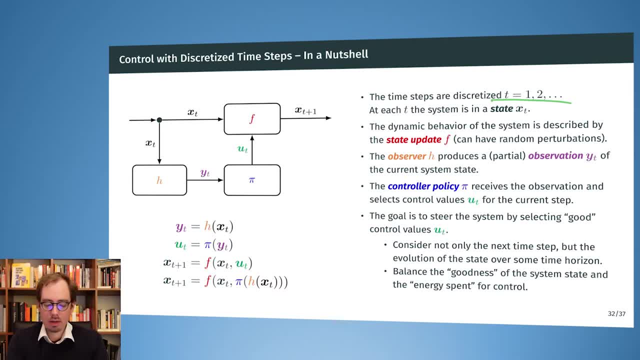 chemical plant or the electrical engine or the inverted pendulum. it has a system state and the system state is described in a vector x au, vector x of t. and also the dimension of this vector x of t depends obviously on on the system itself. so if it has a hundred state components, or or maybe only two, okay, and there is a state. 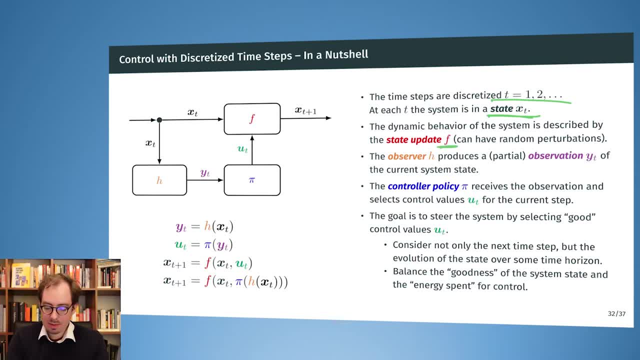 update function f and this state update function. it describes how the system evolves from one time step to the next. so we have our inverted pendulum and if we do nothing then it will start to fall down. and function f: it describes how fast it will the the state of the pendulum will will. 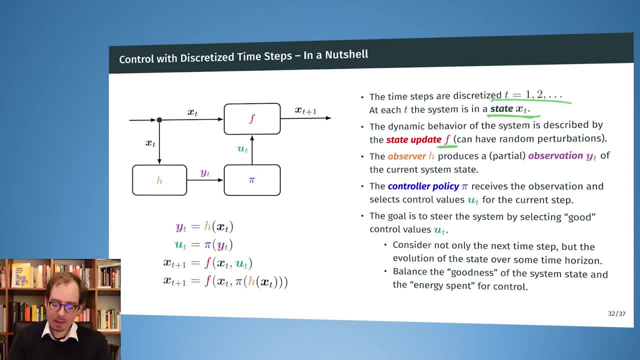 change, but the state. it not only depends on the previous state. so here we have x- t, which is the current time step, and then we go to x, t plus one, so you to the state of the next time step. but we are the the. the dynamics of this are influenced by a. 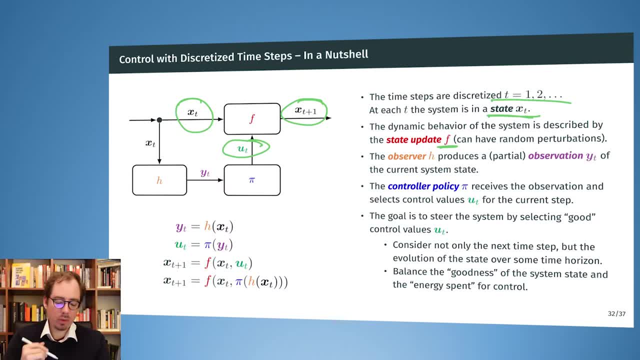 control value that we can choose. so we are controlling the system. so, in addition to the previous state, we are also putting our control influence into the state update and then this produces x t plus one, and here we could also have some randomness involved. but we are not considering this today, or we're not even considering it in this course to have control. 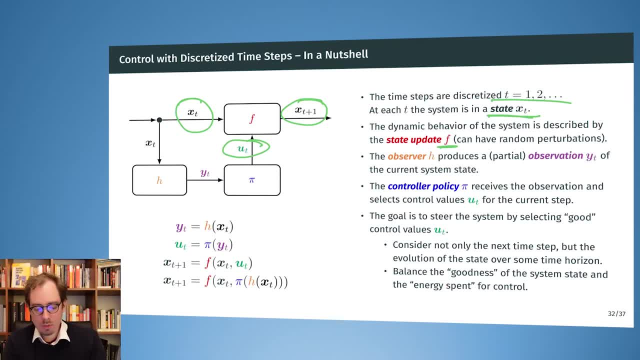 with randomness, okay, but how do we know how to influence? so if we are somehow turning the knobs to control our chemical plant, how do we know in which direction to turn the knobs? we are obviously observing the system. so we have an observer h that sits on top of the system. 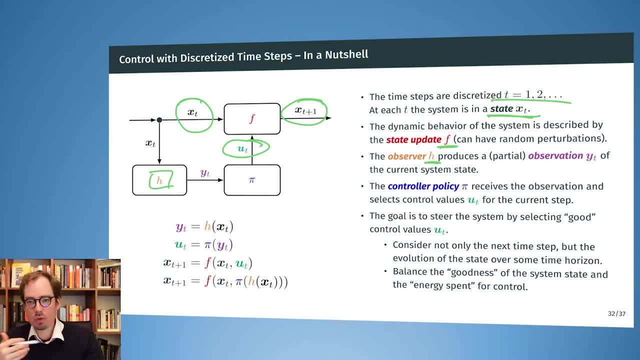 and it gives us a partial or somehow transformed observation coming from the current state of the system. so here we have the current state, x, t, and our observer, it gives us an observation yt, which is somehow derived from that. and then we have a control policy and the control policy tells: 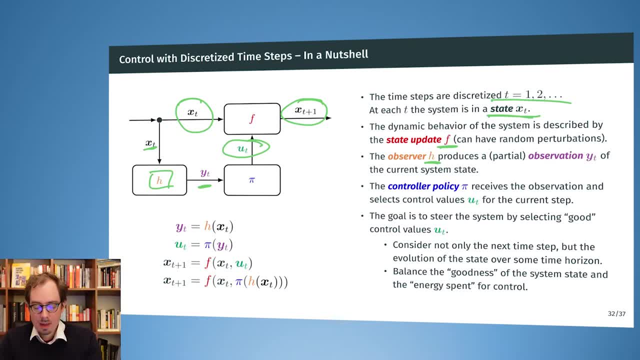 us for which observed system state we are selecting, which control value we are going to get for the as input to impact the state update of our system, and this can be described by the equation here on the on the left hand side. so we have our observation, we 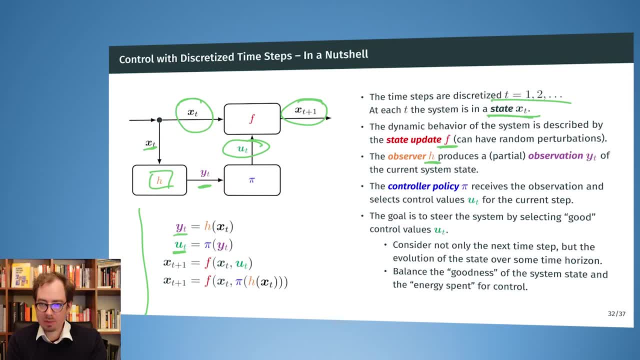 have our control value. as the result of the observation, we put the current state and the control value into the state update to get to the next state, and if we now just plug everyone in, we get one big equation now for the new state update, which again only depends on xt. So here this guy. we can also then write it. 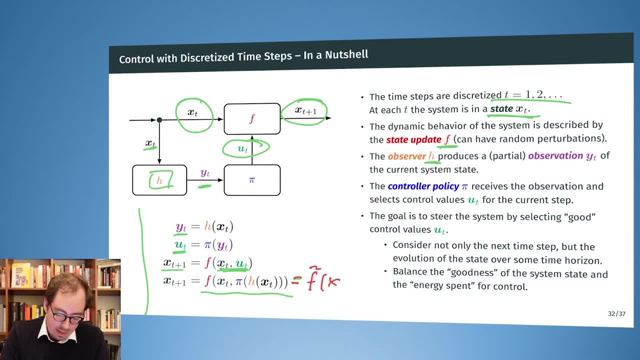 SF tilde of xt, because it only depends on xt and by appropriately selecting the observer and by appropriately selecting the control policy pi, we can create a new system that has a different behavior so our original. if we don't have a control input here, then if the system was left to its own devices. 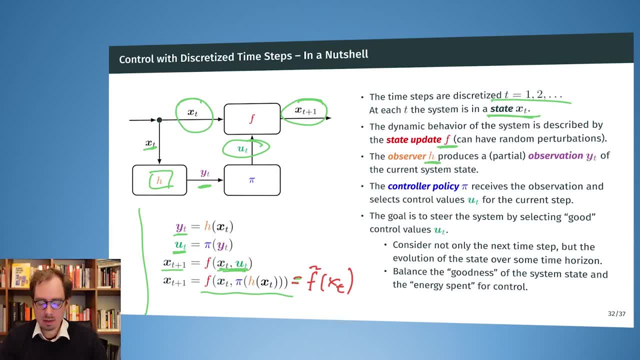 we would have f somehow describing its evolution, and maybe the chemical plant would explode or our inverted pendulum would drop down. but we don't want that. therefore, we are adding the controller and we get a new system that has a new, updated behavior and that is somehow preferable, and so 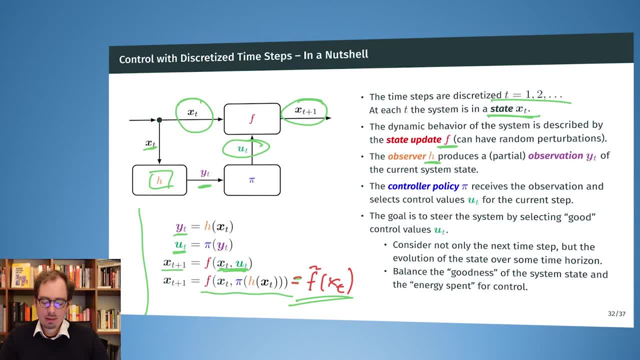 the big question is how to design this controller here. and the controller it should steer the system in a way that it shows good behavior. and what we do in this example is we explicitly model an optimization problem so that the control values selected by the controller are the result of an 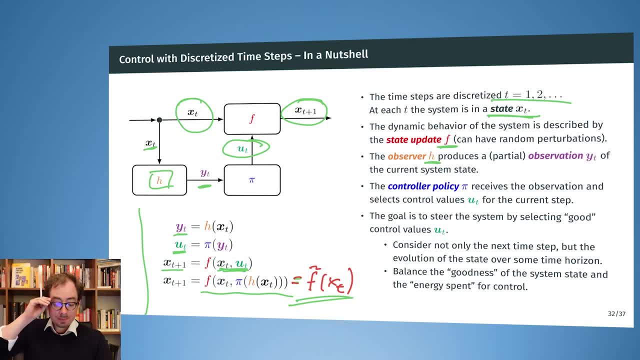 optimization problem, And for that we not only want to consider just the next time- step xt plus 1, but we want to forecast into the future and want to optimize in some time window that is long enough and also want to balance the system state that we achieve. 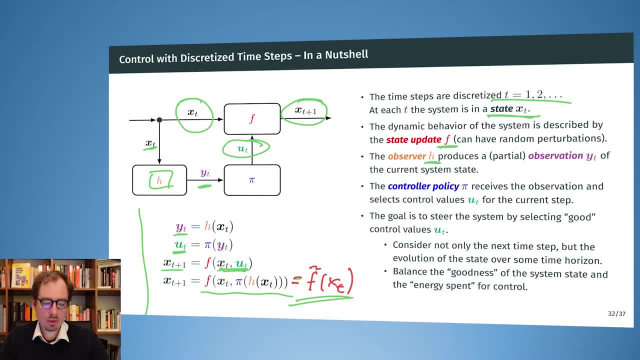 with the energy spent for control. So sometimes we can just put into a million volts into our system to immediately jump back to a good state. but we have to balance and somehow also the energy spent might not be worth a certain improvement in the system state. so somehow there is here also a trade-off. 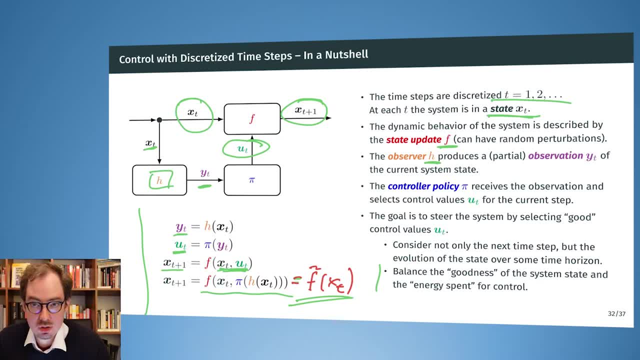 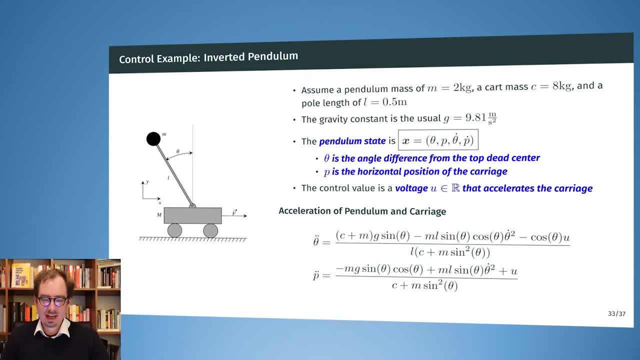 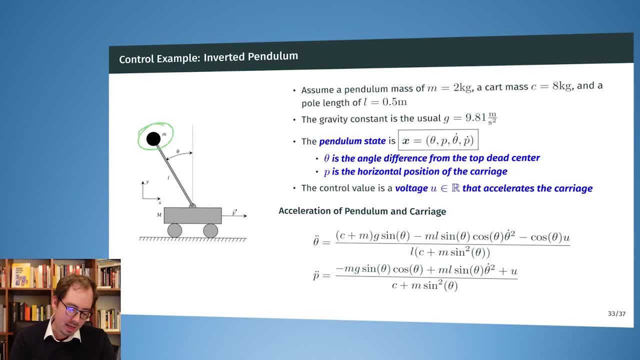 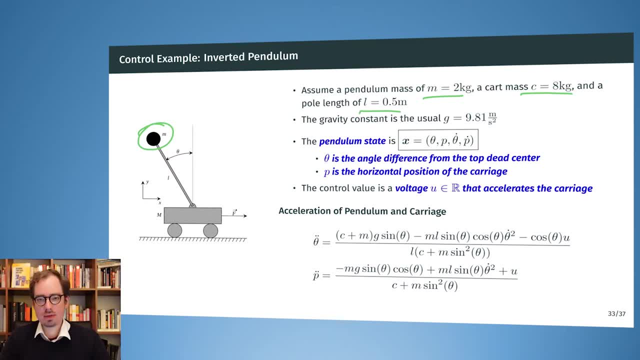 centimeters In addition, the usual gravity constant here on earth. And the first question is: how do we describe the state of the pendulum? and in this case the state vector x will have four components, which is the angle, so the degree here with how much the pendulum is deviating from the upper top. 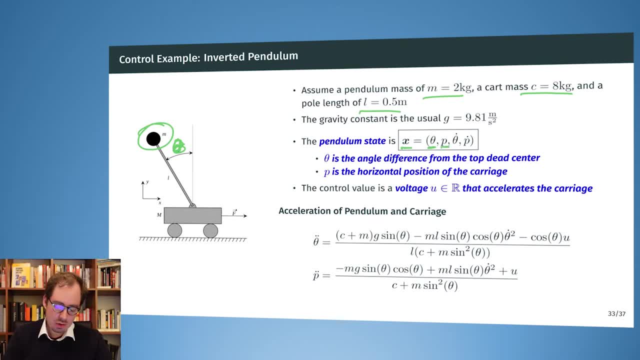 dead center, The position of the carriage. so here this is P, here is the, the position on the horizontal axis where we are with our cart, and in addition also the angle speed and the position speed of the cart, And so the the speed here. 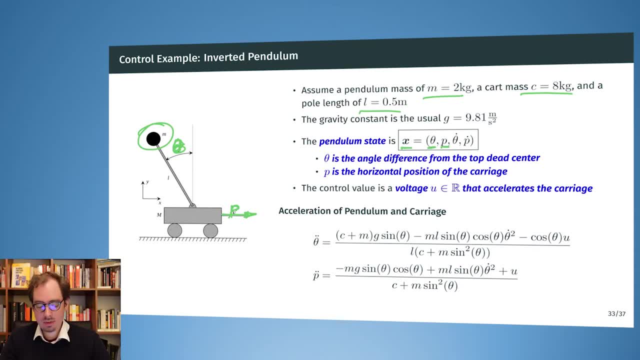 is important because in a physical system there is momentum, and so we have to consider that as well when we want to describe the coming evolution of the system. state: Okay, how can we control? We can apply a certain voltage to the card that will then accelerate it into one or the other. 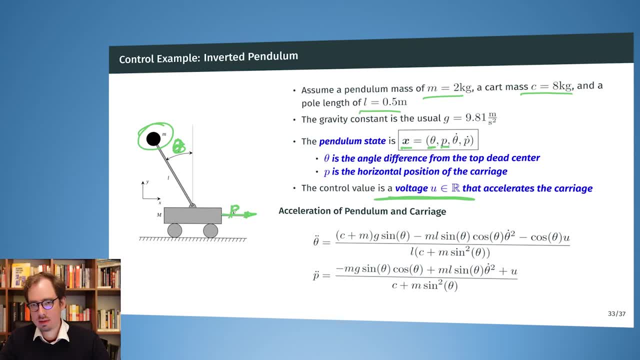 direction. So we cannot immediately set the speed of the card. We can only influence the speed of the card over time by accelerating it, by applying a certain voltage and changing the momentum. And now there are a couple of big, scary equations. Don't look at them too closely. So. 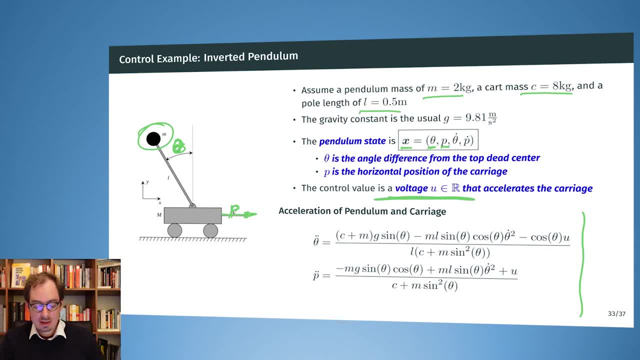 big, scary equations coming from physics that describe the acceleration of the pendulum and the carriage, And this is just the dynamics in the terms of a partial differential equation, or no, it's actually an ordinary differential equation. And well, this is then for a continuous time. this would be the. 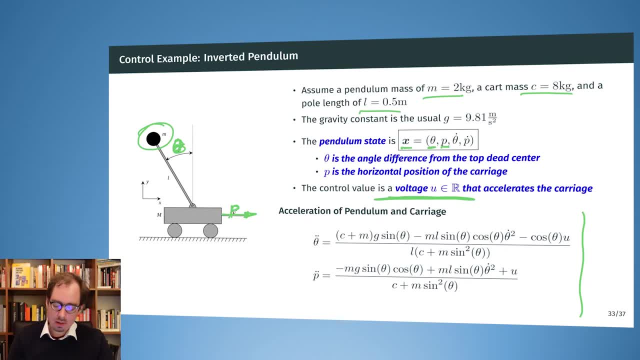 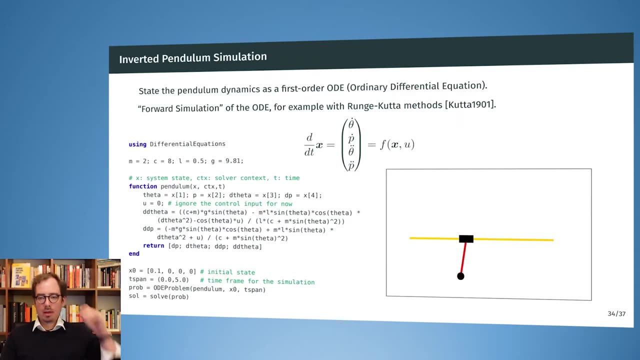 update of the state, because here we are already considering the U, so the control input that we want to select, how that is impacting on the acceleration for the angle And also the position of the card. Okay, So in computer science we can work with simulation, so we don't have to spend weeks and weeks. 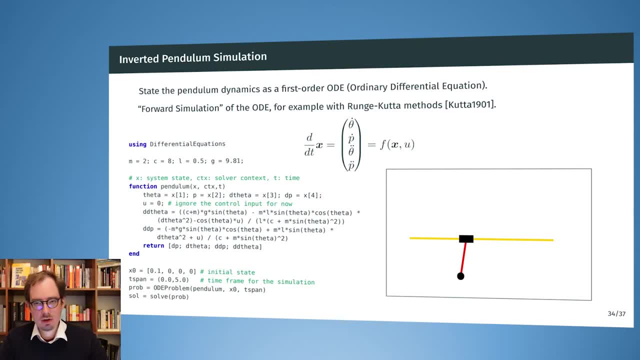 to build up a physical demonstrator, even though that's a lot of fun. but here we are using just a simulation. So the big scary equation, it was put into Julia code down here and we can plug everything into a ODA solver. 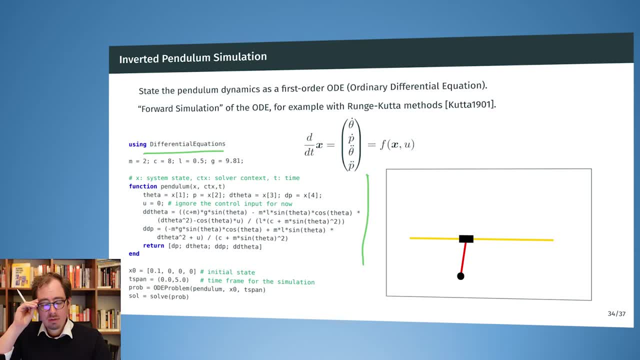 an off-the-shelf ODE solver from the differential equations package, and the only thing that is important here is that we have a way of really precisely predicting what will happen in this idealized world with the inverted pendulum. And if I click on here and if you do that on the 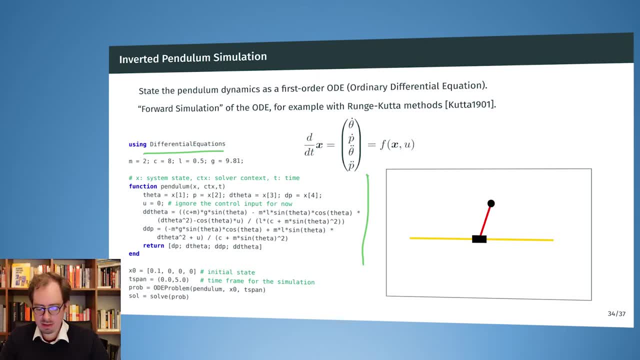 Adobe Reader software. it can show you the animation. I think it requires JavaScript in the PDF reader or something to show the animation, and so you see how the pendulum is swinging. and well, we are obviously so. this is frictionless, so the pendulum will never stop swinging without 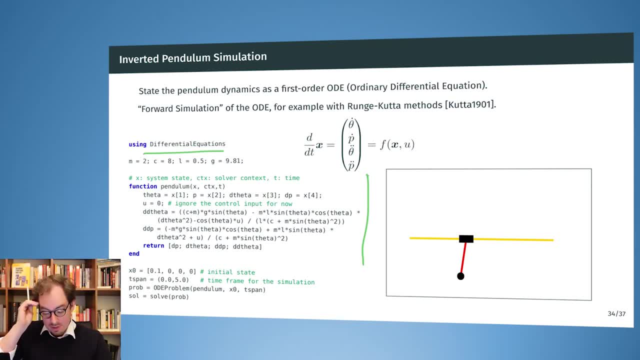 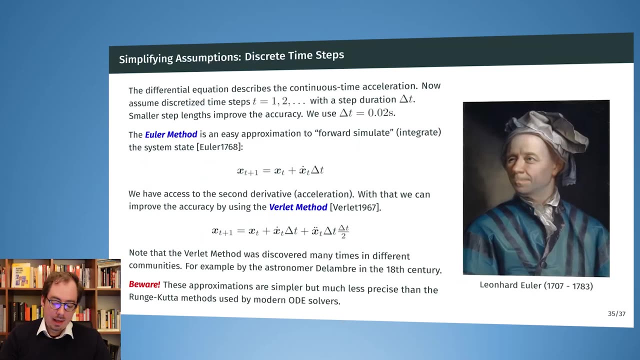 friction. but we are very interested in now changing the movement of the card in a way that the pendulum will swing upright and will also stay upright. How can we do that? first of all, let's see ways to predict the movement of the card. That is less. 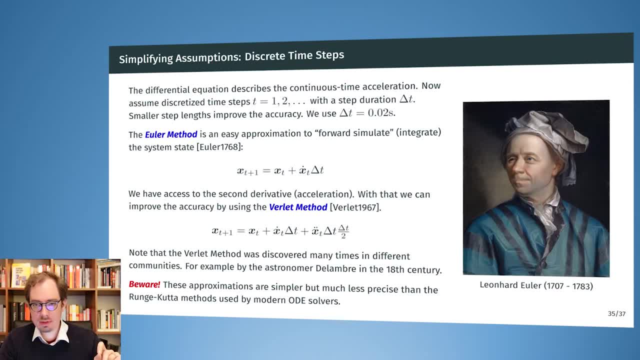 difficult than using the ODE solvers from the differential equations package. So the ODE solvers from the differential equations package. they use something that is derived from the so-called Runge-Kutta methods- pretty, incredibly simple, but still useful for us. Let's see a little bit on the 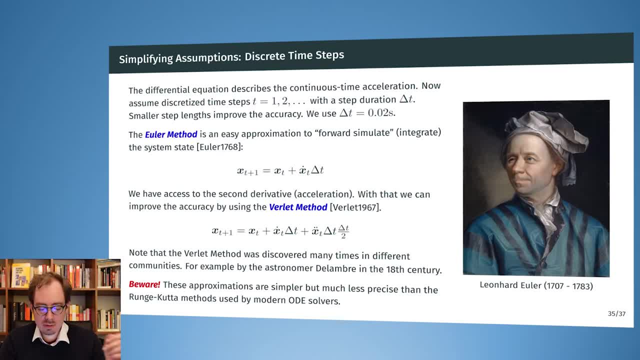 ODE solver that I have just shown you. So this is the ODE solver from the differential equations: Precise, fast, but also pretty involved. Now we will look at a more simple way, and the more simple way is the Euler method. 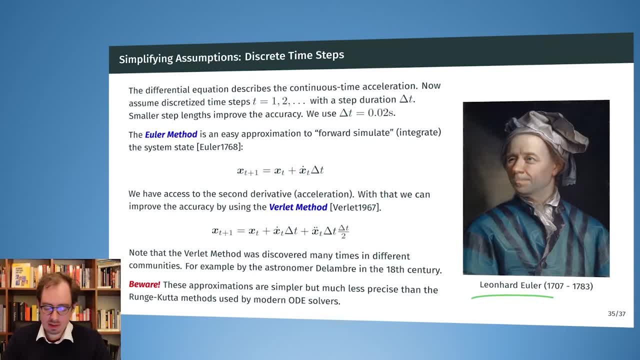 Euler, again famous mathematician, Swiss mathematician from the 17th, from the 18th century, and what he used to do, the integration, or to do the forward simulation, is to just assume constant speed at discrete time steps. so let's say, here we have. 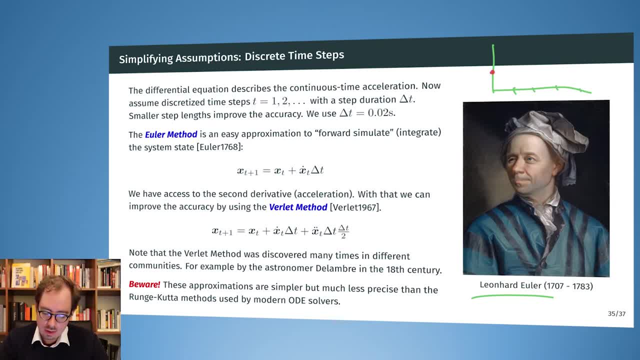 discrete time steps and we have some initial state here and then we just assume constant speed and then at the next time step- maybe speed has changed a little bit- then constant speed, next time step again constant speed, and so on. 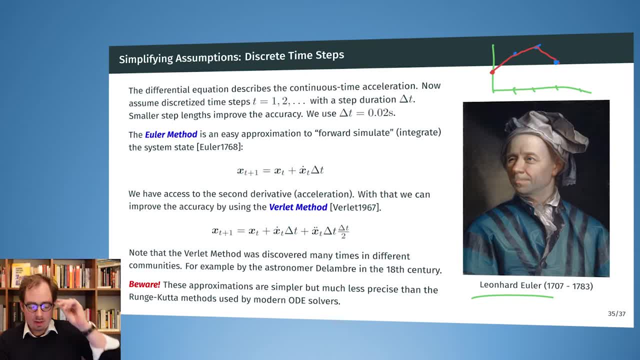 And this is a very, very gross estimate and if you can avoid it, you shouldn't use the Euler method. It's just one of the simplest methods we can use to forward simulate by assuming, at the current time step what's the speed. 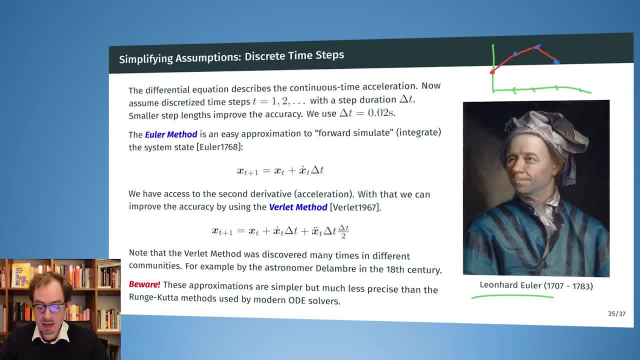 we multiply the change by the time step length and add that on top. So here, Euler method. By having access to the second derivative, we can do a little bit better, a little bit better. this is then called the Verlet method, so a French physicist from the 20th century, and what he says is: 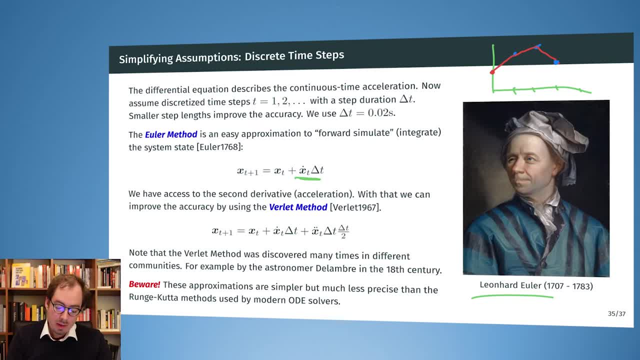 well, if we know the second derivative, then we know by how much we will accelerate in the current time frame. And so we know that we will accelerate if this were a movement. so not everything's a movement, but if this were a movement. 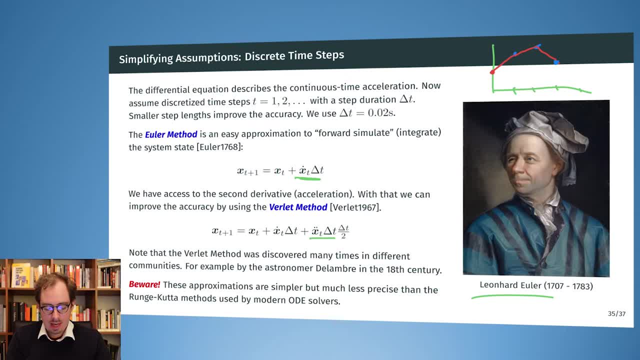 and Xt would be the point. Then Xt is the first derivative in the time domain and dot, dot Xt is the acceleration in the time domain. And then if the acceleration was constant, then we would know that we would accelerate by that much, and then probably you did that already in high school physics, and then we can multiply the acceleration by again. 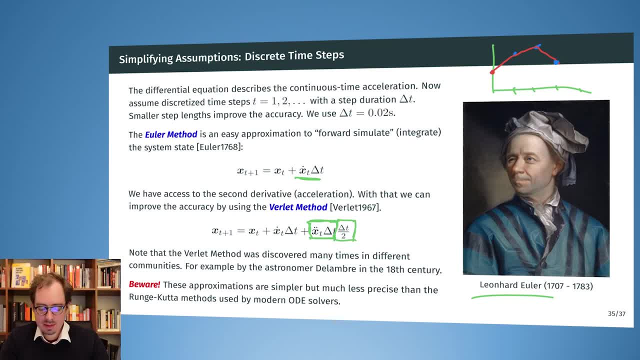 the time step divided by two, And this gives us then the additional difference in position that we gained by acceleration just in that time frame. So somehow, on this axis, here we have then the speed, and then here we have the time frame. 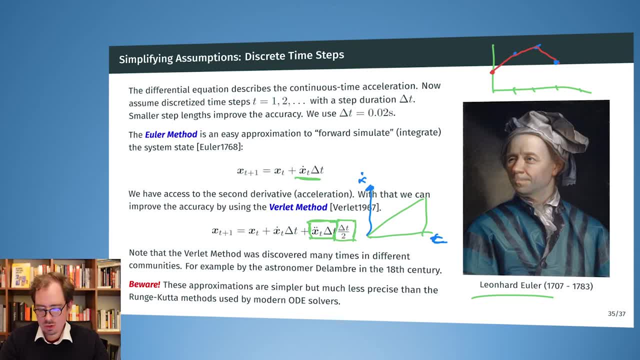 and then we can essentially take the integral of this triangle here to say: what is the difference, in position already, from the current acceleration in this time step? And well, this assumes that acceleration is constant, which is also not true in general in these differential equations. 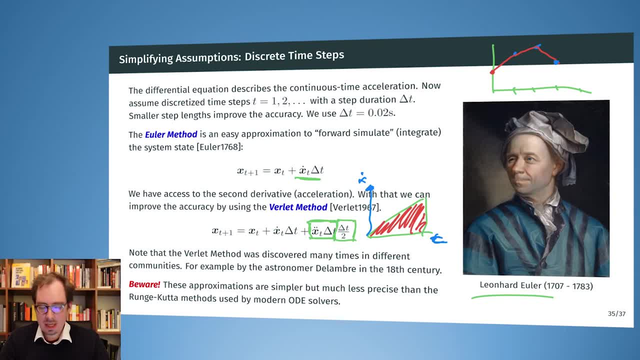 even within such a time step. But when we make the time step, then we know that acceleration is constant. When we make the time steps smaller and smaller and smaller, somehow this will become a predictor. that is already a lot better than just using the Euler method. 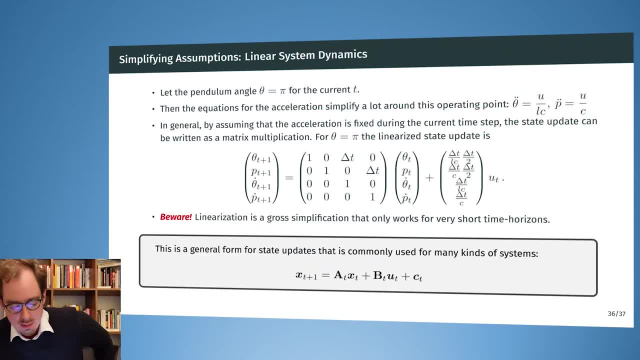 Okay, but why are we interested in the Euler method? The question is: how can we pose the control problem as an optimization problem, And for that we already need to do a forward simulation For several time steps as part of our optimization that we are doing. 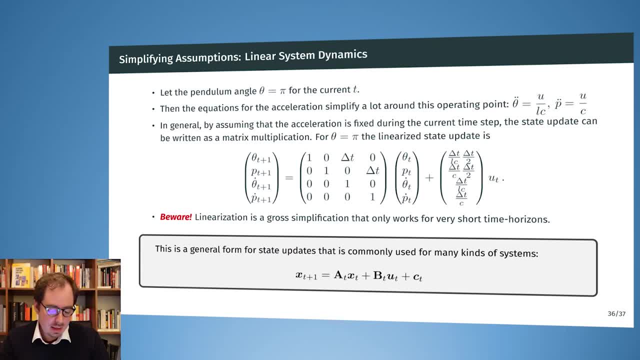 Okay, but in addition to just assuming discrete time steps, we want to linearize the system dynamics in every time step. Let's assume that the angle of our cart or the angle of the pendulum is pi, So the pendulum is pi. 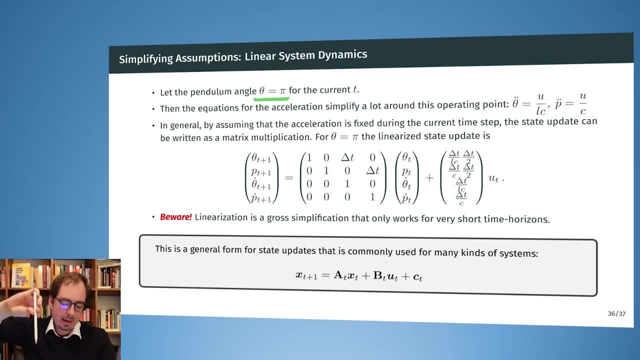 The pendulum is pointing down And the pendulum angle is exactly pi at the current time, step t that we consider. And if that is the case, then all of these scary equations that we saw, they are simplifying quite a lot, because then the acceleration will be just u. 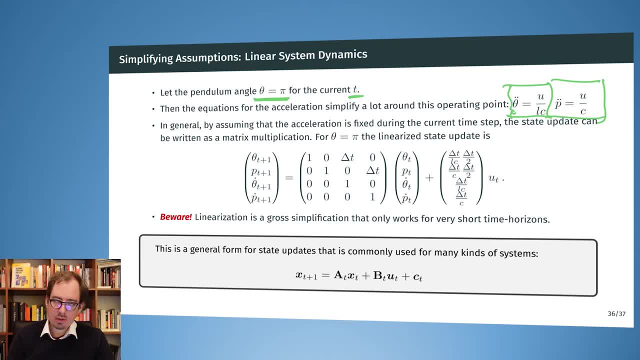 so our control divided by LC- the acceleration of the pendulum angle and the acceleration of the cart position- is just u divided by Lc, And so this already looks a little bit simpler. Obviously, this will be again a scary equation when pi is a little bit different. 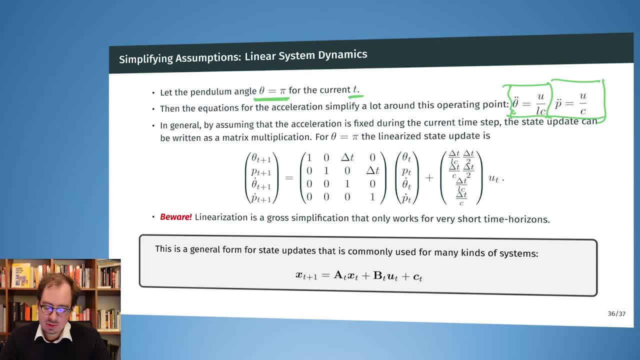 But let's just take this for an example, because it will make our equation for the x position here a little bit easier to work with. So we assume now from the Verlet method that the acceleration is fixed during the current time step. 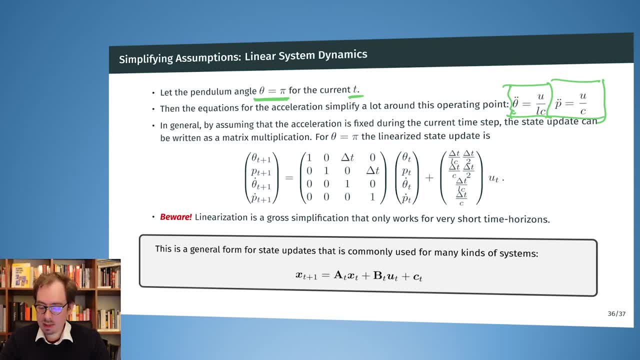 And we have here computed the current acceleration by the two equations that you saw up here. And now we can write down the state update: so our f, So we have x is f. And this guy. we can write down the following: So we have our next state. 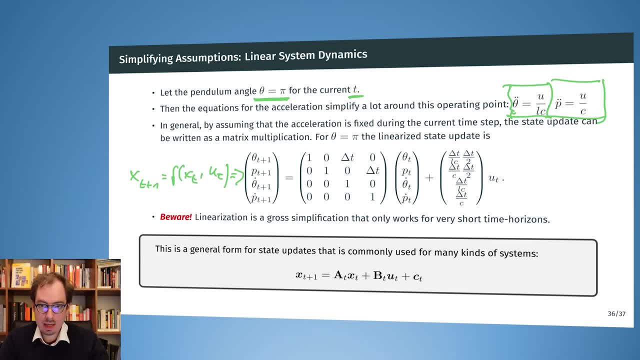 so with the angle, the position and the speed And the state update, it can be written by doing just matrix vector multiplications. So let's look only at the first line here. So the first line here, at the next angle, And I'm doing it down here because I have more space- 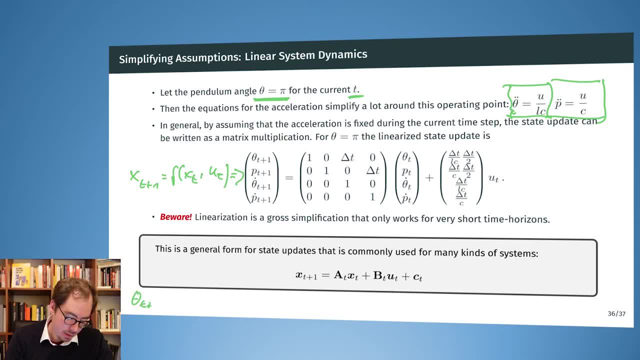 So here, essentially, the first line translates as the following: So the next angle will be one times the angle from the last time step, of the current time step plus the current speed times, the duration of the time step plus. and now we come to Verlet's method. 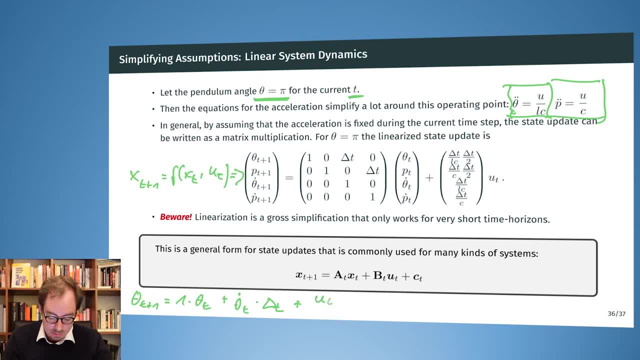 Here then we have ut, so the control value, the voltage that we apply, divided by lc times the time step, times the time step divided by two. So this will be probably pretty small, because here we have two times or we have the time duration of the step squared. 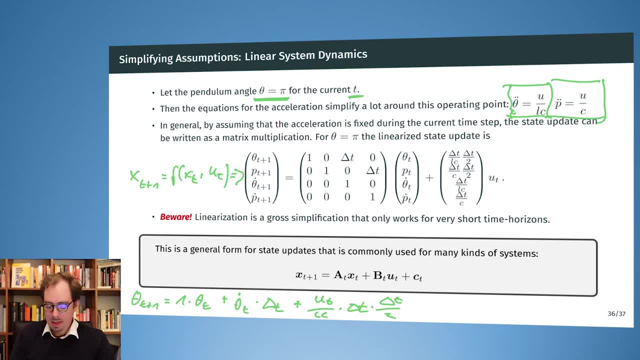 But you see that here we exactly end up with the equation for the Verlet method, And it's pretty simple because in the end it's just the matrix vector multiplication, And here we can describe not only the update of the angle but the update for the entire state of our system. 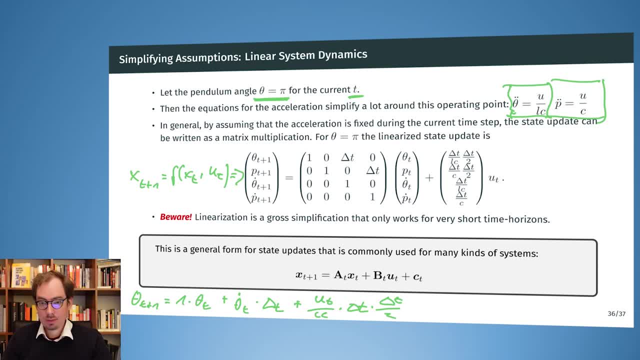 by just doing matrix vector multiplication. So the same here is then also true for the change in speed, So the change in speed of the angle. So here we would first have so of t plus one, here we would have first the current speed. 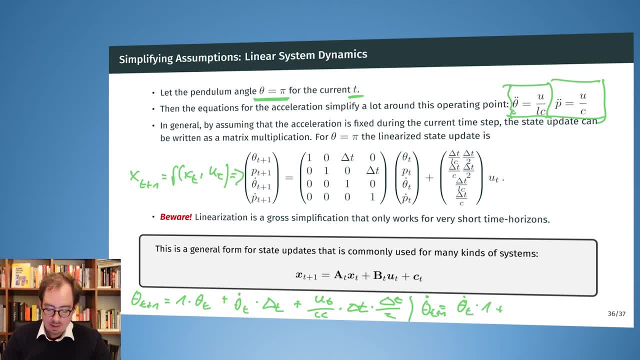 one times plus and plus. and now here we have ut divided by lc times, the step duration, And again here. this is just the first discretized and then linearized state update for our system, So we have arrived at a very general form. 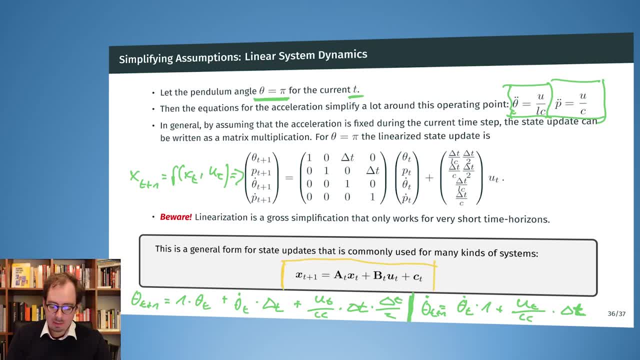 that is used for describing many, many, many different kinds of systems. So first discretizing the time domain and then linearizing. but notice that here the matrices, they will be different for the different time steps. So if we can already foresee, 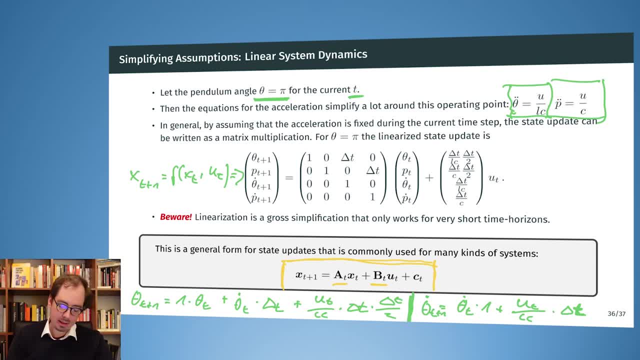 the future evolution we can here modify that the at will be matching. Okay, And now what we do is we are stacking these state updates, Because when we have a way to compute xt plus one from xt and ut, then we can do that also for multiple steps. 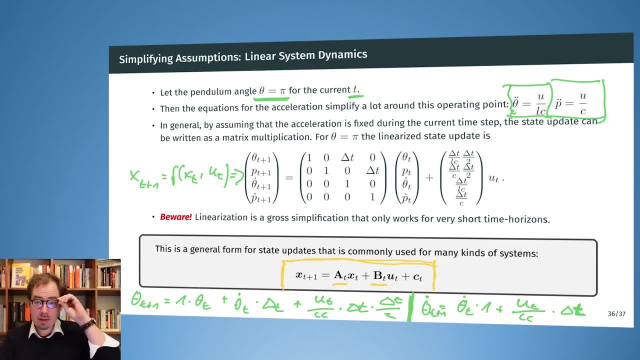 into the future and then also compute xt plus five and so on, And we have a way to describe the evolution of our system depending only on the initial state and afterwards on our control input. And what we then do is we are stacking the state updates. 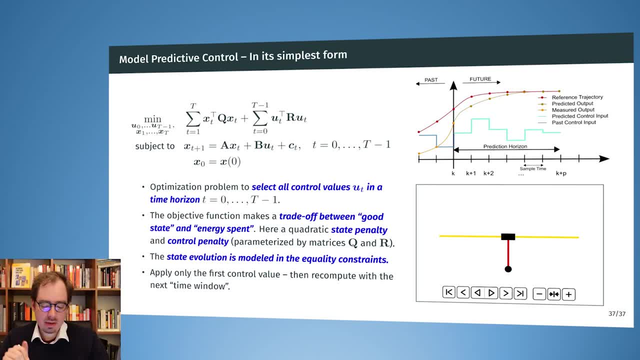 and putting the result or putting the resulting equation as an equality constraint of our optimization problem. So now we are at the heart and probably the most difficult slide. So now what we are doing is called model predictive control, And model predictive control was invented by people. 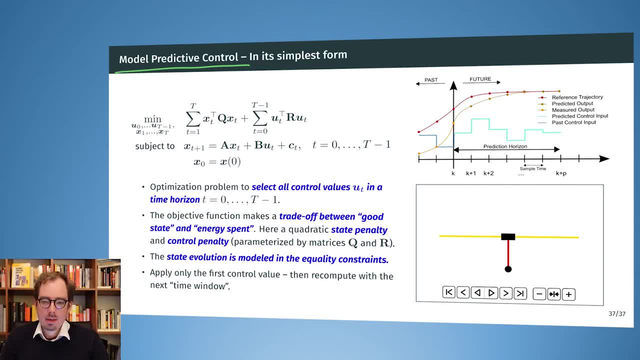 such as Manfred Moragli and others- So, for example, Mr Ben Porath- And they started developing that already in the 70s, when computers were very slow, And back then model predictive control could only be applied to slow moving systems. 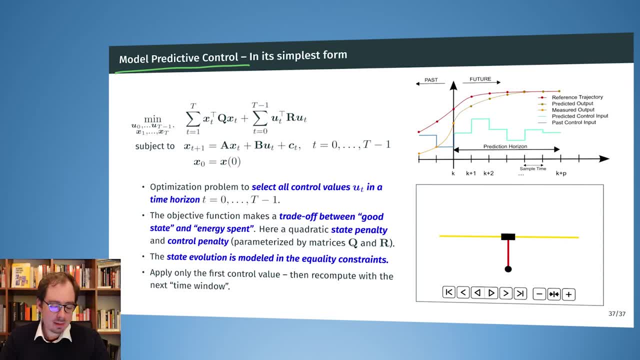 like chemical plants. But today model predictive control is everywhere. It's in your car, It's planes, trains and automobiles. Every physical system that needs good control probably uses some sort of model predictive control, or will soon. So this is really taking over. 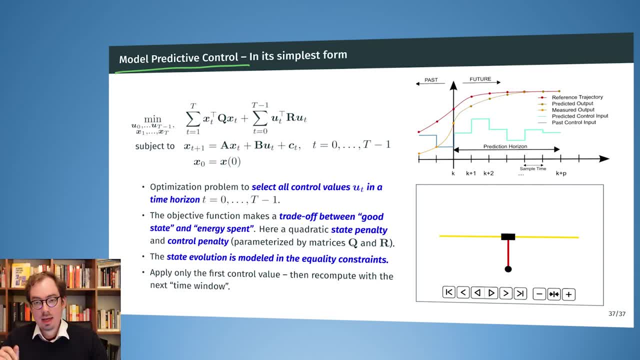 And in model predictive control. what they do is they solve an optimization problem with a very high frequency today. So in your car, if you have an MPC controller somewhere, or in your future autonomous car, this is solving optimization problems hundreds and thousands of times. 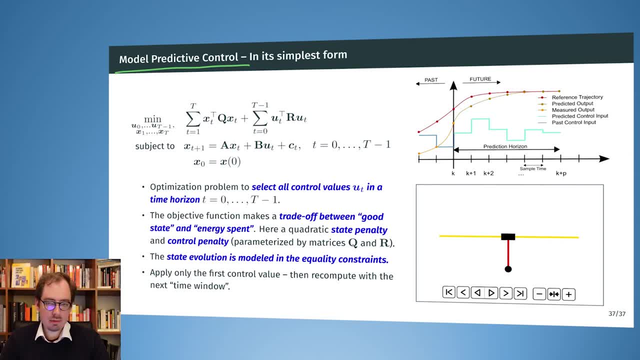 every second and is using the result of the optimization- problem of the optimization- to apply control to steer your car to the middle of the lane and similar things. So obviously today, autonomous driving, they're also using neural networks and they work fine. We don't know. 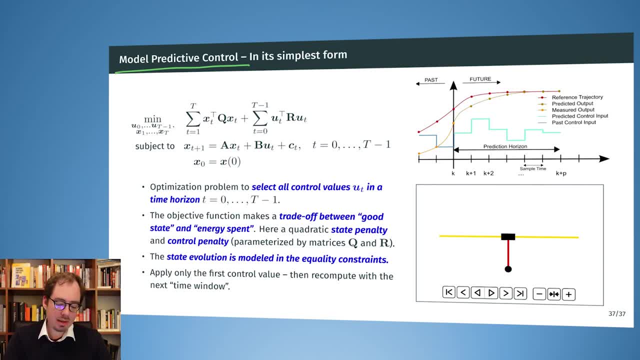 maybe some of the limits, but what you see here, this is the classic engineering approach to do control And over the last 50 years they have developed methods also to describe the limits. So by taking some assumptions on the system and the surrounding environment, 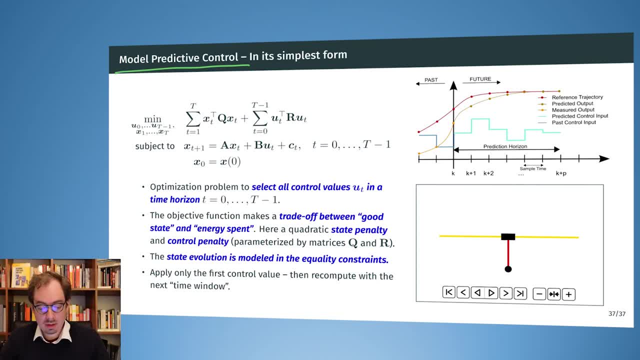 you can then also compute hard limits of what your system will do and what it won't do, And so somehow now there is like a clash between the traditional approaches that include model predictive control, and now neural networks taking over also for like safety critical tasks. 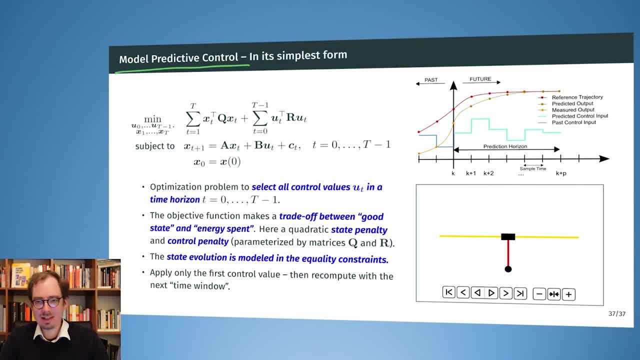 And well, this of course has the patina of many years of development and experience and the tools to also talk about safety critical systems. But what is the optimization problem? What we have to do is we have to simulate our system over several steps into the future. 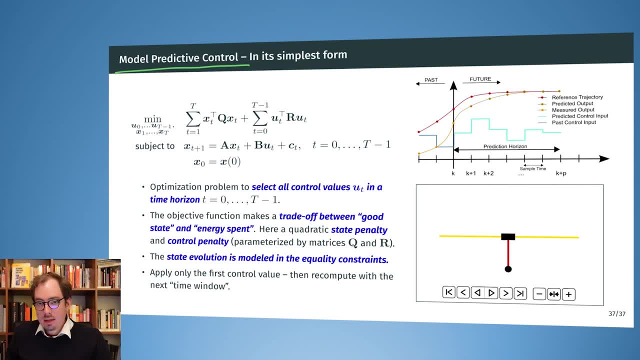 and then do a trade off between the system state- how much do we like the system state- and the control. so the voltage or some other control input that we had to spend in order to achieve that system state. So what we are doing is we have an optimization problem. 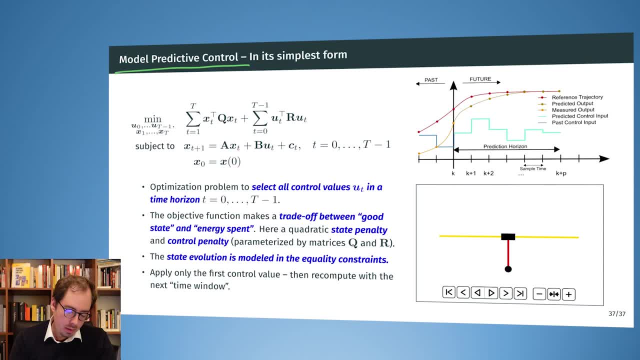 and we are minimizing. We are minimizing overall the control values over a time window and the time window goes from now to some big T, or big T is only a scalar in this case. So sorry about the notation confusion. So this is an optimization problem. 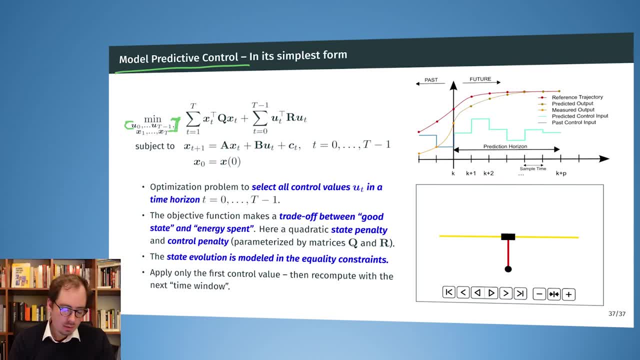 over all the control values, and all the control values here can also be vectors, So we can have also several control values being selected for every time step. Okay, So we are optimizing to find the control values over the entire time horizon up to big T. 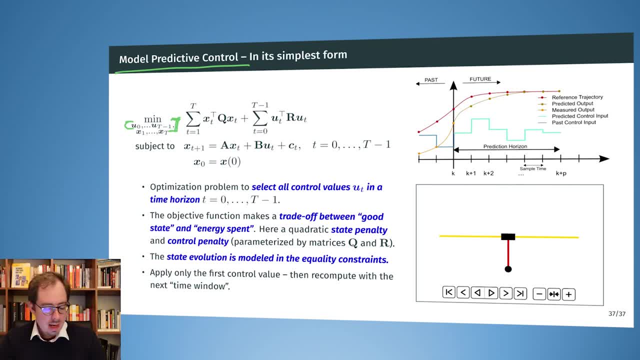 So big T is like 100 or something like that, And in addition, we also consider the states, namely from the next state up to the state at time. big T. However, these are only auxiliary variables, So and these are required to be part of our optimization problem. 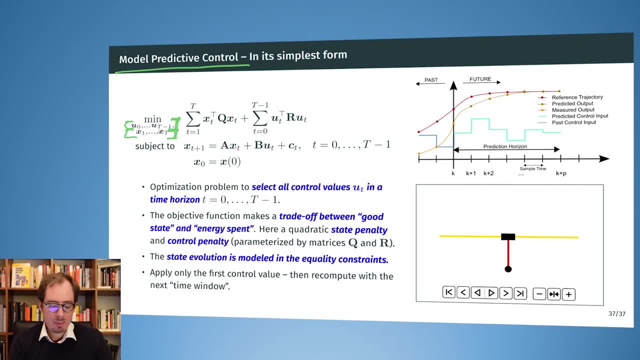 But these here are heavily constrained by an equality constraint that we put Meaning for every state up to from one state to the next. here we put in the equality constraint. that is exactly the kind of state update equations that we saw on the previous slide with the inverted pendulum. 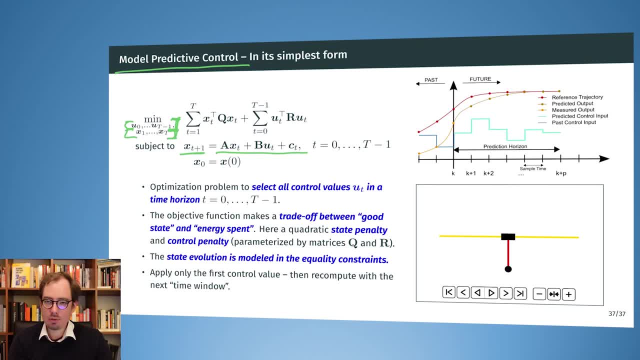 And so we have here some degrees of freedom, but the degrees of freedom exist only in the control values that we can select, Because also the very first system state here this is predetermined, because this comes from the measurement. Here we assume that we entirely know. 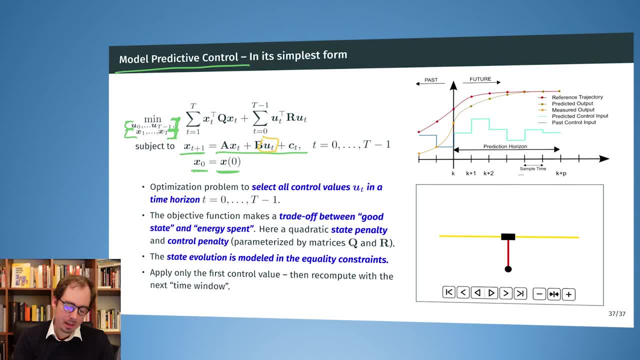 the initial system state. But in this equality constraints here we are doing our simulation. So for the predictive part of model predictive control, this is the predictive part And now we are minimizing to find a good trade-off between the system state that is achieved. 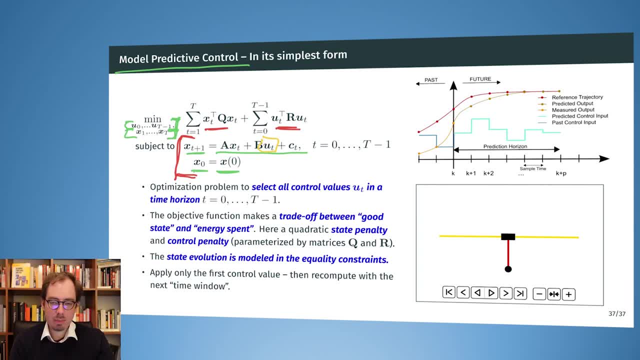 and the control state that has to be spent in order to achieve that state. And there are many variations of that where we have different additional constraints and the constraints are changing over time, because maybe if we are thinking about optimally heating a house, then maybe you have the constraint 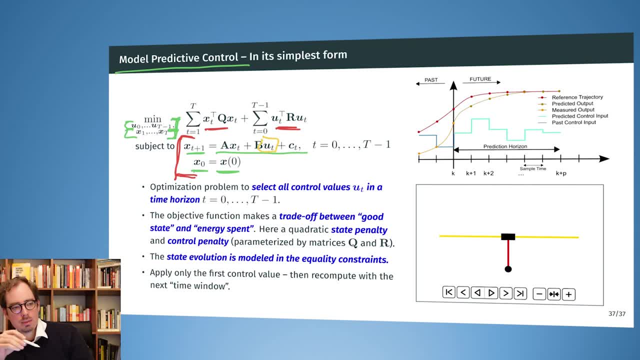 that during the day you need a temperature in the house between- if it's an office- between- 18 and 20 degrees, But at night you don't care. And then, if you formulate the optimization problem, we can have additional constraints and different constraints. 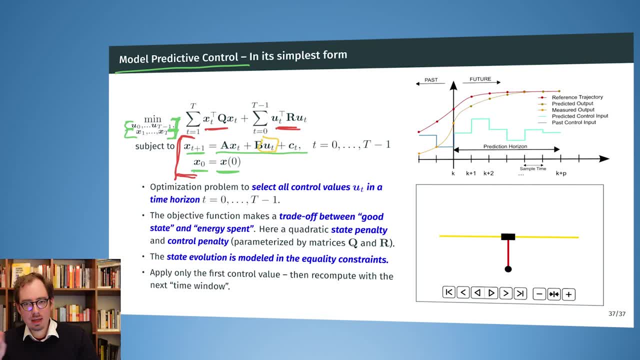 for the different time steps where we say only during the day we have a temperature constraint, at night we don't care, And then by computing optimal heating of the house you can consider when you have to start heating to exactly hit the 18 degrees. 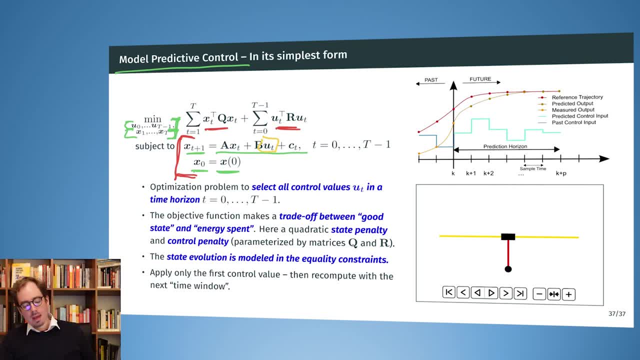 when people arrive early in the morning and things like that. Many variations, also considering then uncertainty. then it's called robust MPC. This is just a playground for good ideas and for important and expensive system where you can have a real impact by optimizing results and not by just having some funky heuristics. 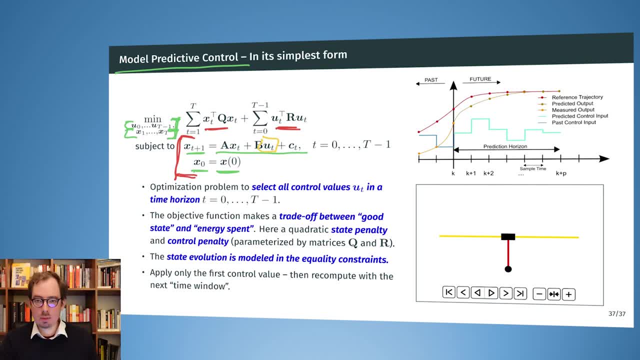 or maybe inexperienced humans that have to do the decision making. So, overall, what MPC then does is considering a time window. So here we have a time window and within this time window we make our prediction. We optimize for the best control values for every time step. 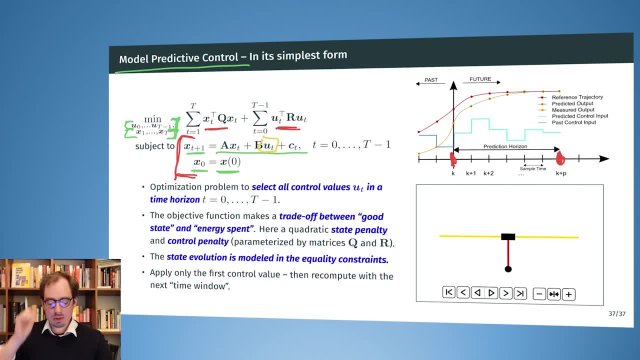 in that prediction horizon and get back a result with the U for every time step here. But what we then do is we apply the control for the first time step, Then we observe what happens. We get a new state observation and then we shift the time window. 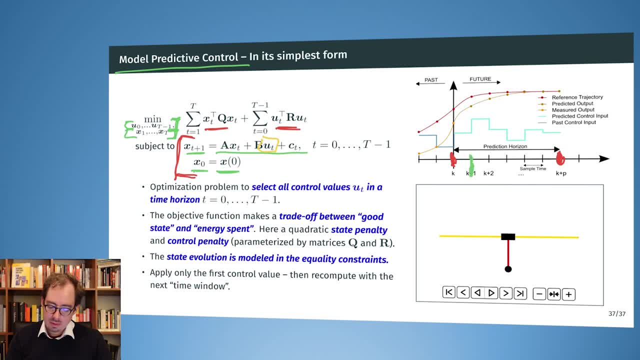 and now we have a second time window that goes from here to here, because the wall clock time has also moved forward, And then we redo the entire optimization for the new time window based on the new state measurements that we got. So we make the prediction. 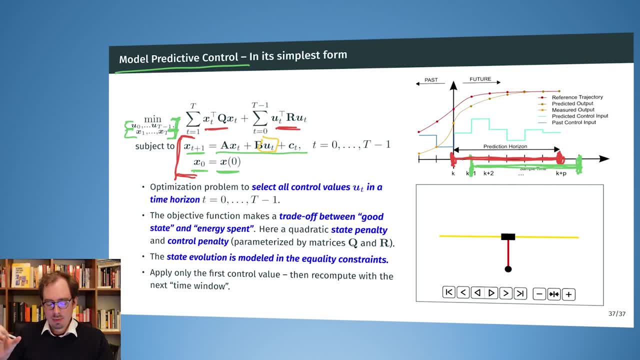 for a long horizon, but we always only apply the result for the first time step, And that way we can also deal with random influences, because if there is a random influence and the next state measurement is not where we have predicted it, then we can still react. 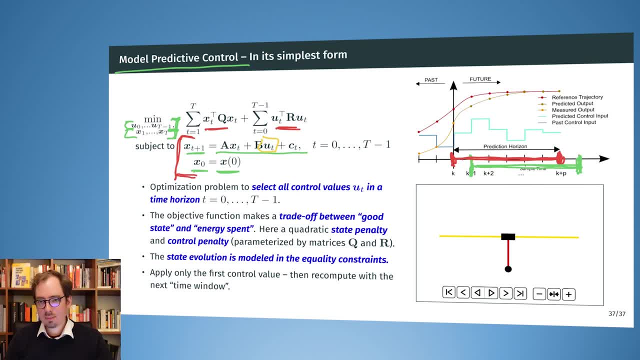 And also our prediction model doesn't have to be perfect, because we are redoing the computation and we can- basically we can- counteract the prediction errors in the next time step when we have updated state measurements. This is the basic idea of model predictive control. 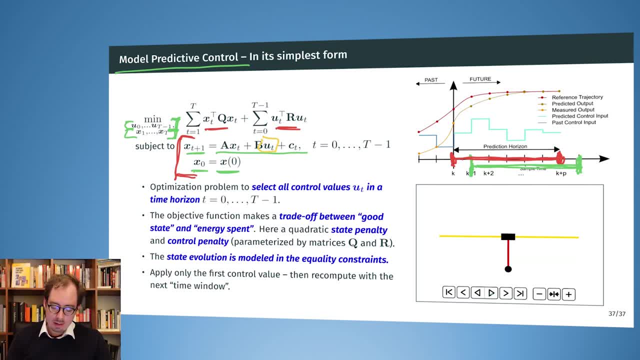 And now applied to our pendulum. if you have the Adobe Reader, you can click on the play button to see the animation. I think we can also put it into the video here. You see that the pendulum- it starts moving and there is a swing up of the pendulum. 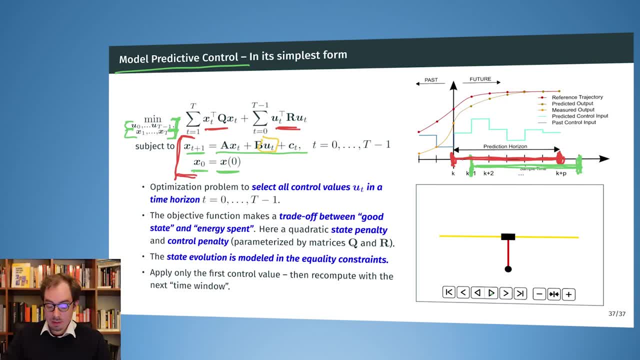 and the pendulum is actually kept upright. So here for this very small example, we see that the controller actually has found a strategy to swing up the pendulum, And in the exercises you will be then deriving your own controller and we will treat a different system. 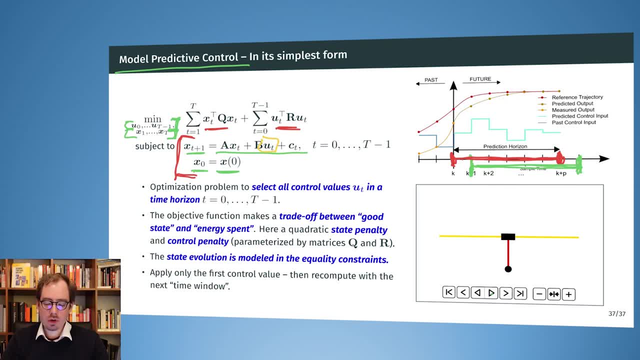 but there you will also be able to force a new behavior on your system, that to do something it wouldn't normally do, like for the pendulum to stay exactly upright. With that we conclude today's lecture. So this was more about applications, and these will be applications. 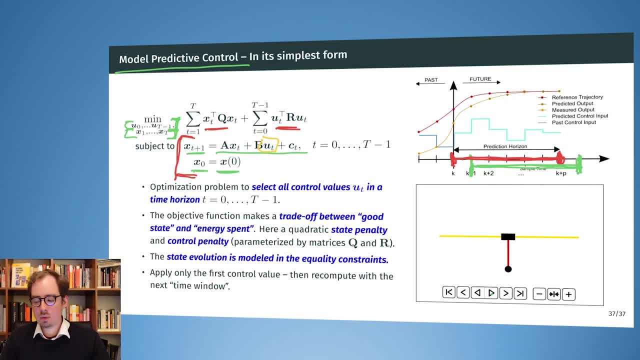 that will follow us into the coming weeks with the exercises. So here we try to cover a wide range of topics to see what optimization can do, to also see what are the different tricks that have been applied or developed in the different domains, and also to give you 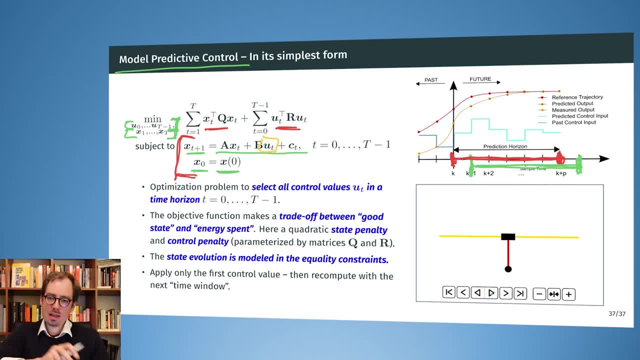 a sense of the possibilities to do: optimization in space, optimization in time, optimization in space and time and maybe many other application examples that you will encounter in the future, either in this course or later in your professional work.